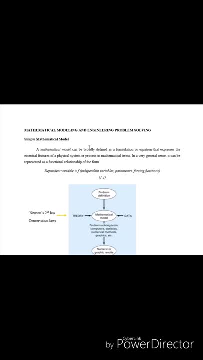 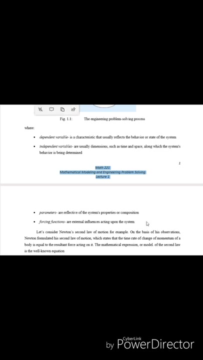 Assalamu alaikum and good day class. So obviously this is our first lecture or first discussion in math 2 to 1, or mathematical solutions for civil engineering problems. Okay, so obviously in this discussion, what we are about to discuss has something to do with mathematical modeling. 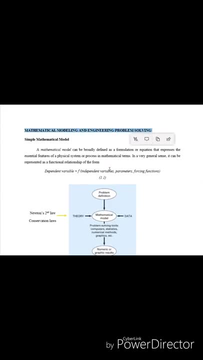 and engineering problem solving. Okay, so in broader sense, or let's, if you're to talk about the overview of this discussion. Our discussion for this, for this, at this moment, is about the concept behind mathematical modeling, or we will be defining some terminologies At the same time. 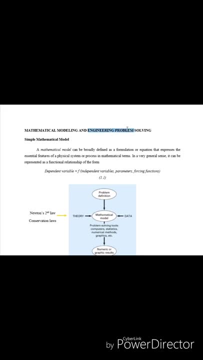 I will be introducing to you on how to solve problem solving involving engineering or involving the field of engineering. Okay, so bear with this video as we are about to discuss, or as we are about to do, to introduce. what is this subject and what involves to solve. 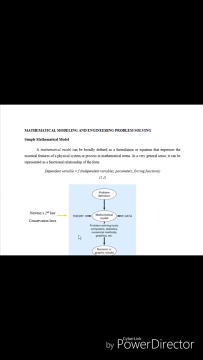 engineering problems. So let's get started, So let's get started, So let's get started certain problems involving engineering problems. Okay, so, with that being said, first let's define what is a mathematical modeling in its formal definition. Okay, from your lecture, from your 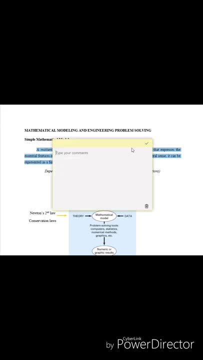 handouts. a mathematical model can broadly defined as a formulation or equation that expresses the essential features of a physical system or process in mathematical terms. But before anything else, I would like to say that you have to download the file that I have uploaded. Okay, same goes for you. 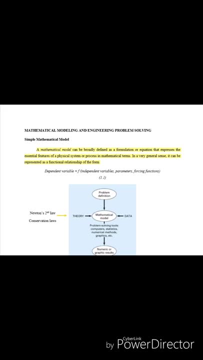 In this lecture one make sure that you have downloaded the file that I have uploaded or that I have posted in our IDMODO classroom. At the same time, I highly encourage that you better print the file that I have uploaded, because that will serve as your outline for you to easily cope up. 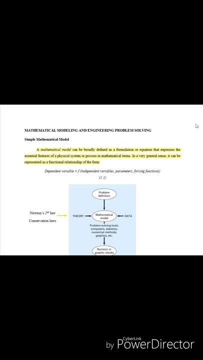 or for you to easily follow While I am discussing this lecture. Okay, I hope I am making myself clear. So, at the same time, if you have any further questions, or if you have clarifications, suggestions or whatever there is or there are, just kindly comment down. 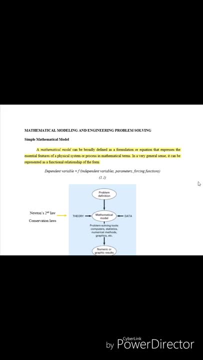 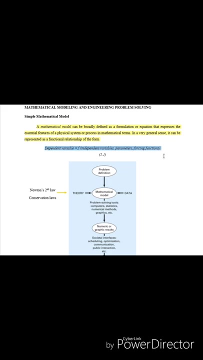 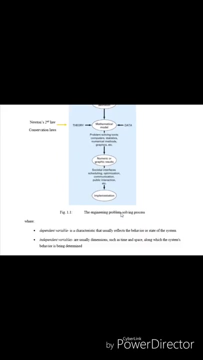 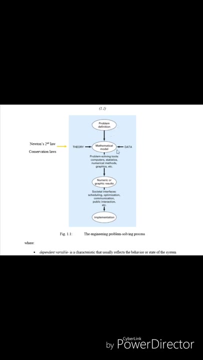 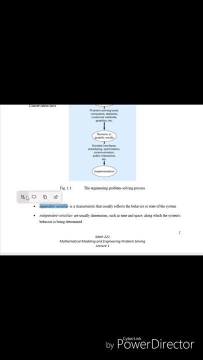 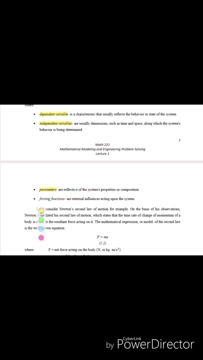 below in your comment section. So let's continue, Let's define mathematical modeling, as I said earlier. Thank you very much for your attention and I will see you in the next lecture. Subtitles by the Amaraorg community- wwwamaraorg. Subtitles by the Amaraorg community. 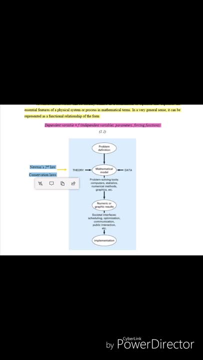 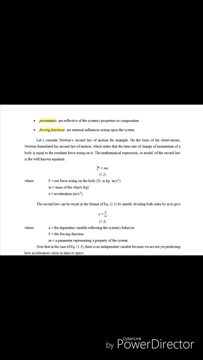 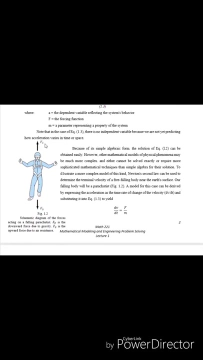 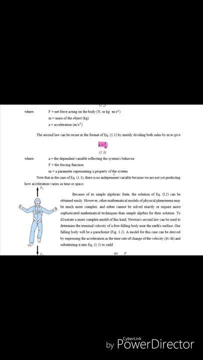 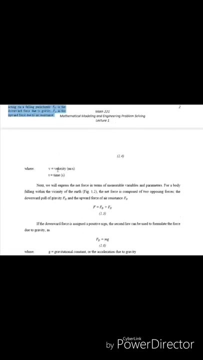 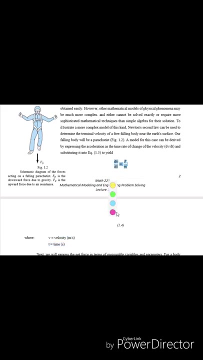 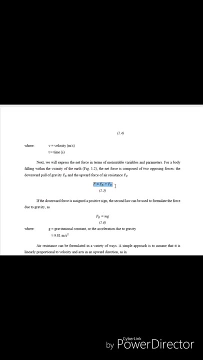 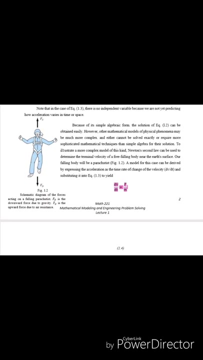 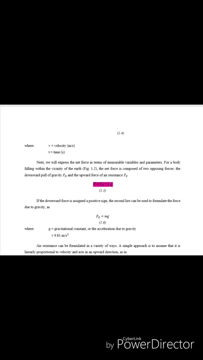 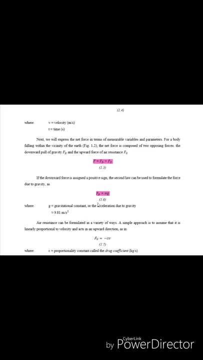 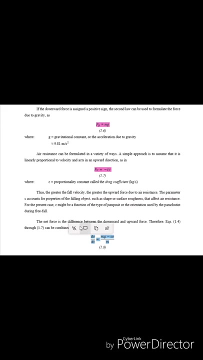 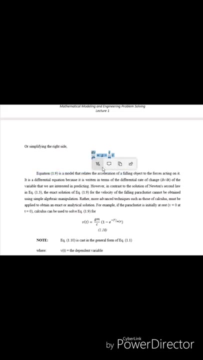 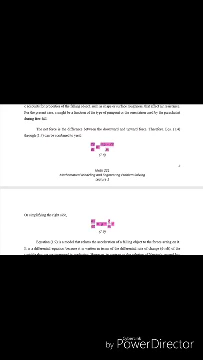 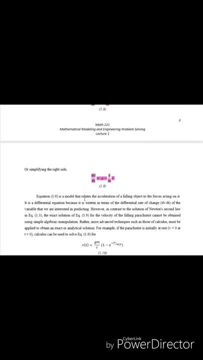 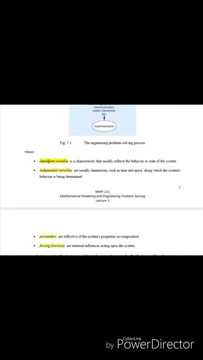 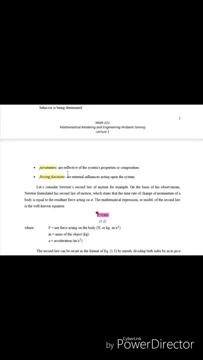 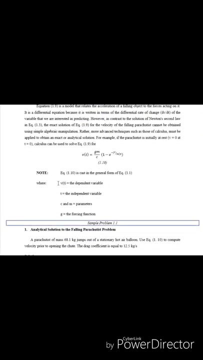 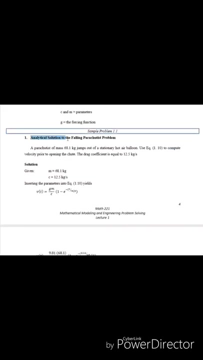 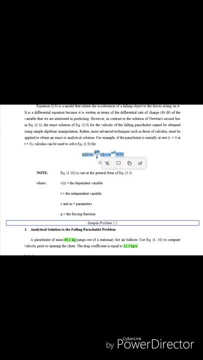 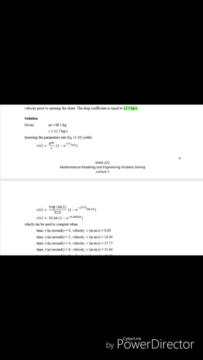 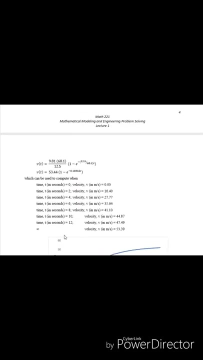 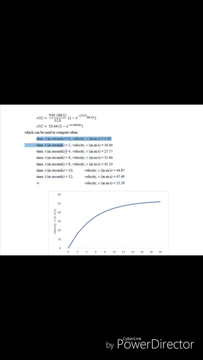 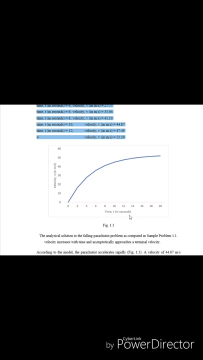